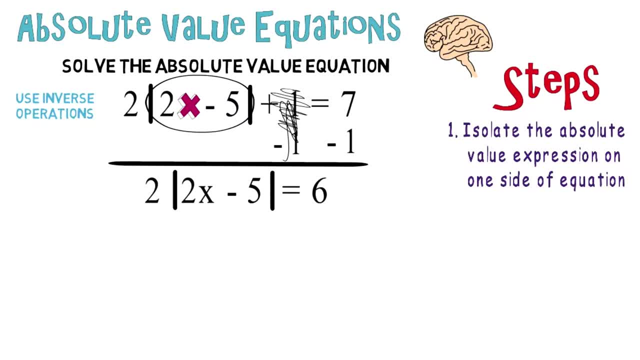 2x minus 5 equals 6.. And again, we want to use inverse operations. So let's divide both sides by 2.. Divide by 2.. Divide by 2.. 2 and 2 cancel each other out, And then you're left with the following absolute value of 2x minus. 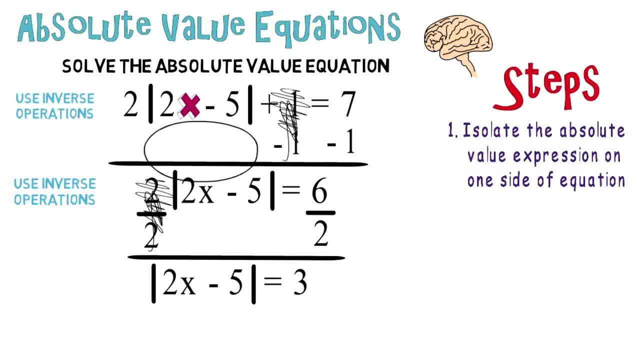 5 equals 3.. Notice: the absolute value is isolated. The absolute value expression is isolated, So we can check off step one and move on to step two. Step two: If the expression equals a negative number, then it's a no solution. So let's take 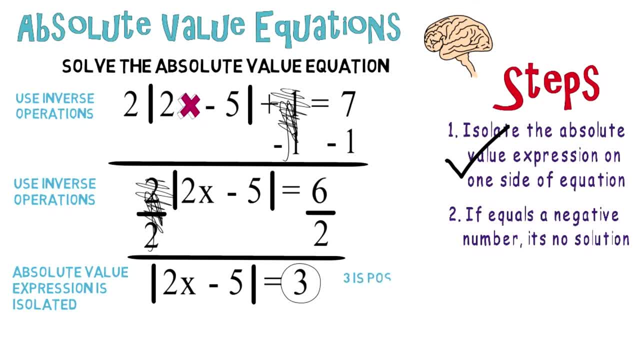 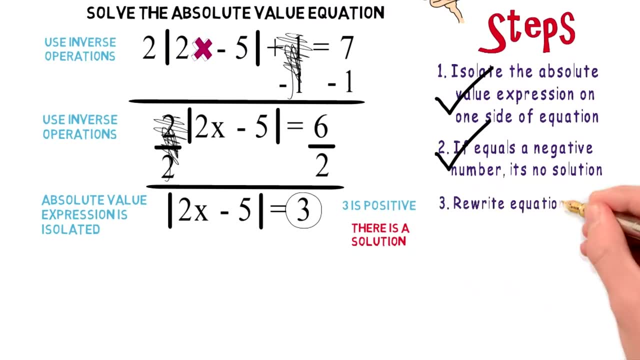 a look here: It equals positive 3.. 3 is a positive number, So there is a solution. So now we're going to check off step number two and go on to step number three, which is rewrite equations as one positive and one negative solution. 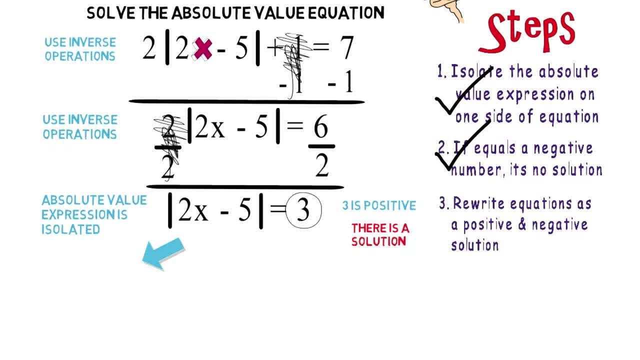 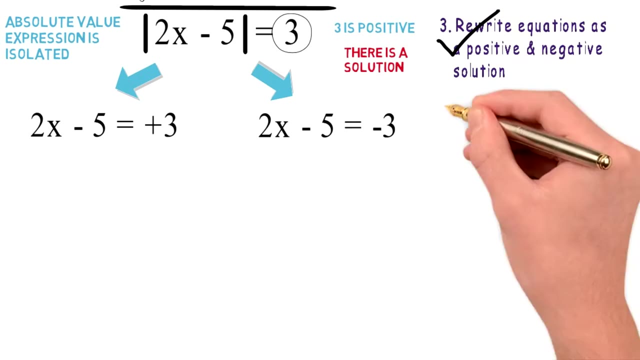 solution. So, for example, let's separate into a positive solution: 2x minus five equals three. Let's also separate into a negative solution: 2x minus five equals negative three. We can then check off step number three and move on to step number four, which is solve. 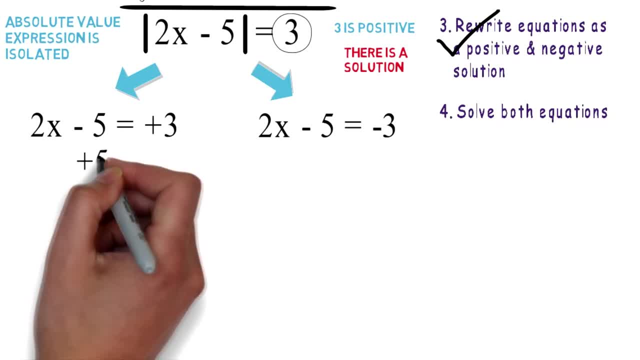 both equations, So let's do that. We're going to use inverse operations, So let's add five to both sides of the equation. Positive five and negative five will cancel out And you're left with 2x equals eight. Again, you want to use inverse operations, So let's divide. 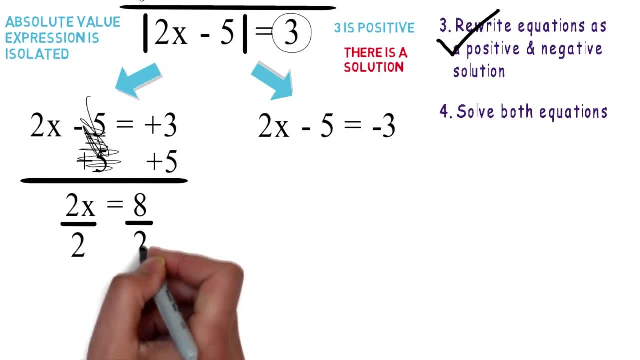 by two to both sides of the equation: Positive two, negative two cancel each other out And you're left with x equals four. Now we have to do the same thing to our other equation. Add five to both sides of the equation. Positive five and negative five cancel each other out.